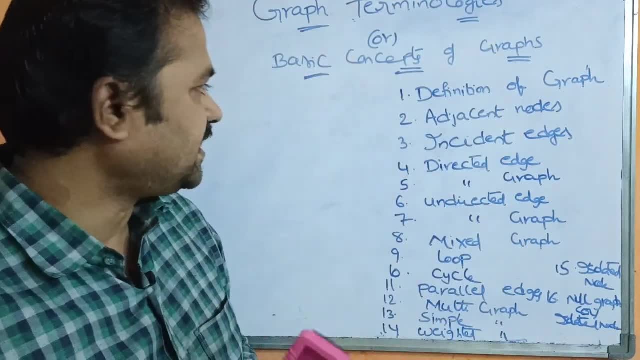 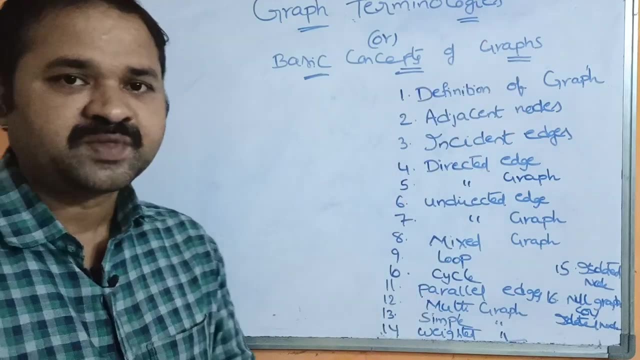 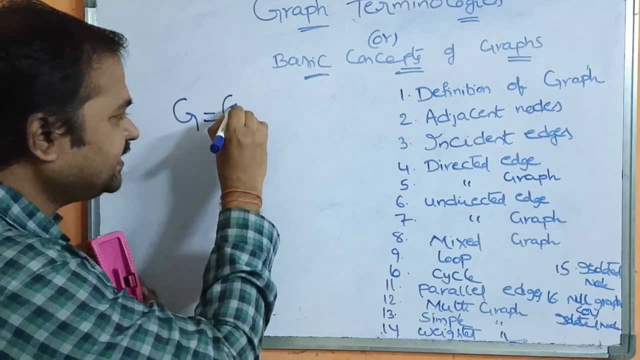 same, only So in this class. in this video, we are going to discuss about these 16 terminologies. First, let us see the first terminology: Definition of a graph. A graph is defined by using g, So g is equal to. it is defined by a pair called v comma e, where v represents 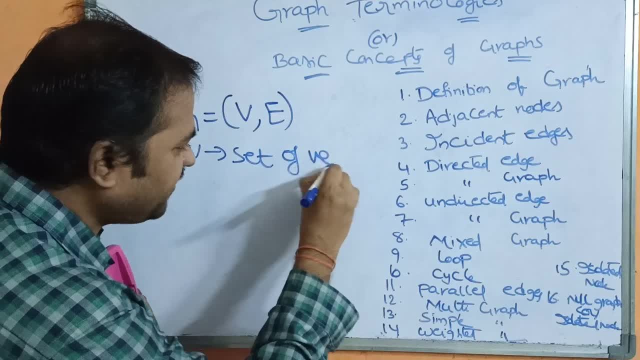 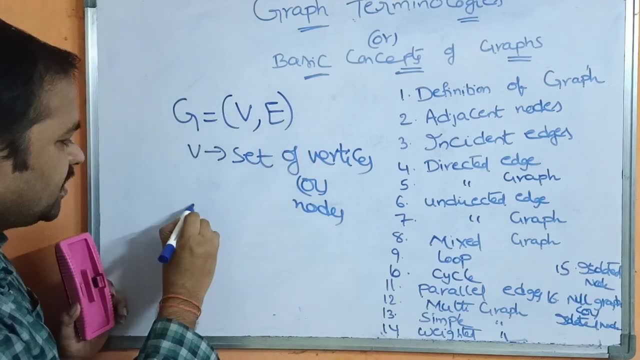 a set of vertices. v stands for vertices. We can call vertices as vertices. We can call vertices as vertices. We can call vertices as vertices. We can call nodes also. So set of vertices are nodes And e represents a set of edges, E represents 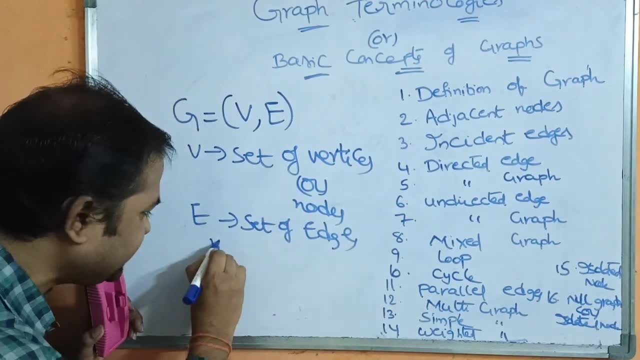 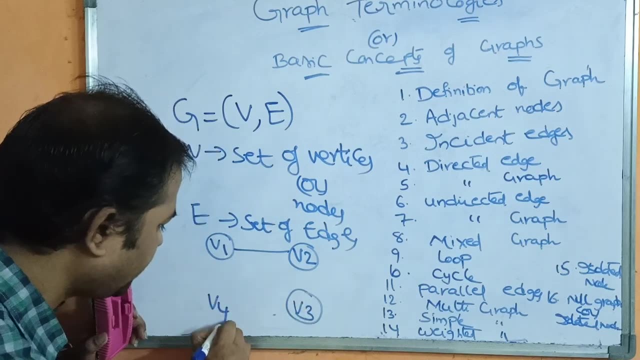 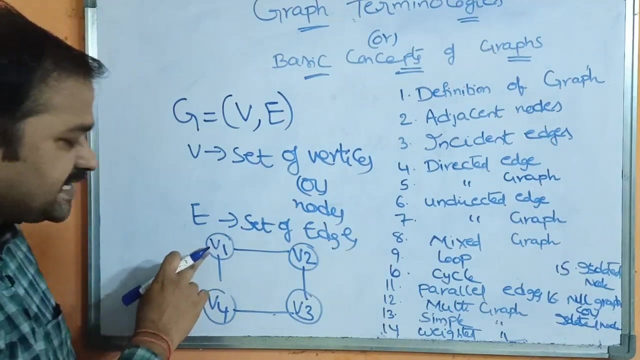 set of edges. Let we have a graph like this: So v1, v2, v3, v4.. So v1, v2, v3, v4. Okay, So in this example, vertices or nodes are nothing but v1, v2, v3, v4. So v is equal to. 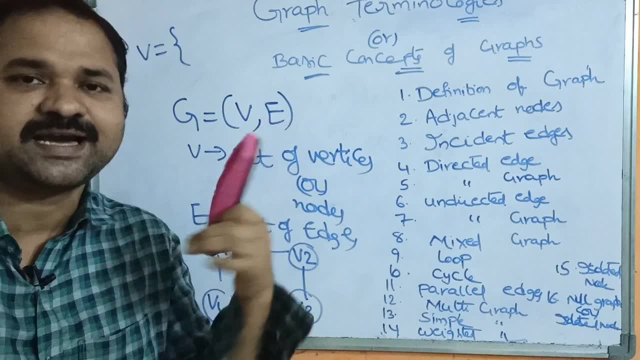 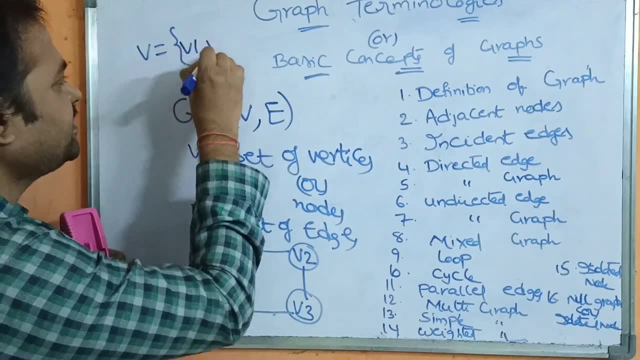 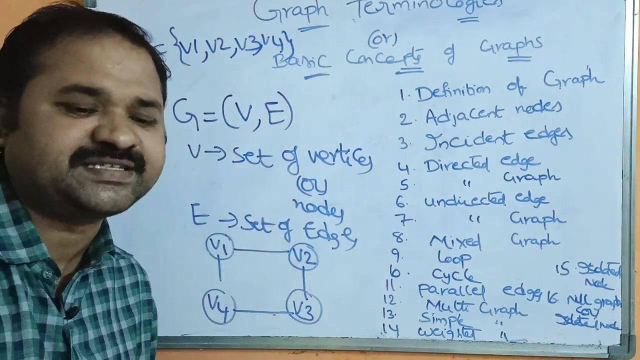 set means we have to place the vertices. Set means a collection of elements which are enclosed in curly braces. So here, what are the vertices? v1 comma, v2 comma, v3 comma, v4.. So this is nothing. but what is v Set of vertices? And the second one is edges. So let this. 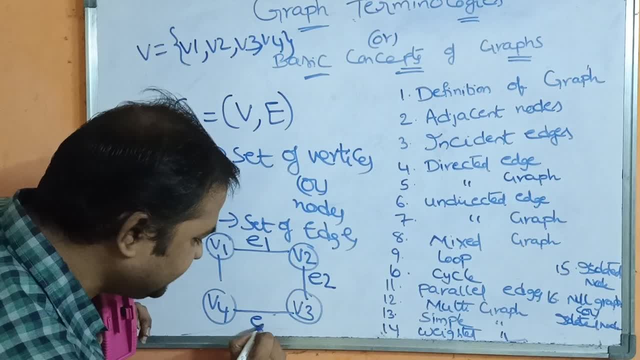 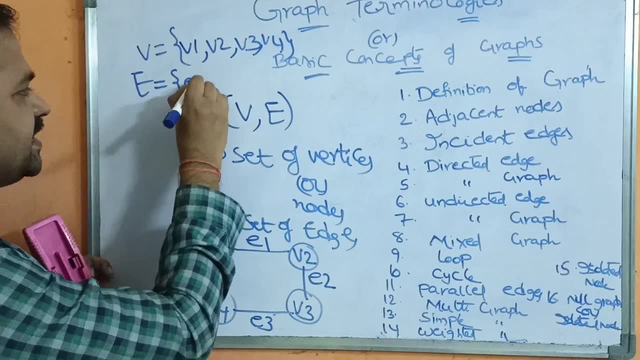 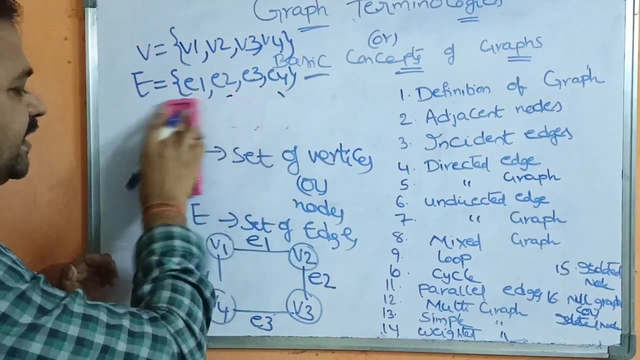 edge is e1.. Let this edge is e2.. Let this edge is e3.. Let this edge is e4.. So e is equal. So e1 comma, e2 comma, e3 comma, e4.. Okay, So what is e1?? e1 is nothing but an edge. 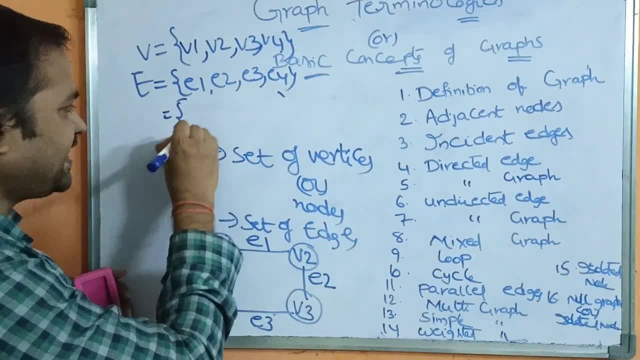 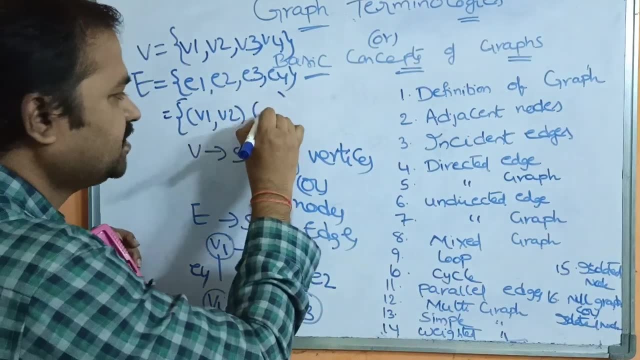 between v1 and v2.. Or we can define like this: So v1 comma v2.. Next, what is e2? An edge between v2 and v3. So we can denote like this: So v2 comma v3.. Next, e3 means an. 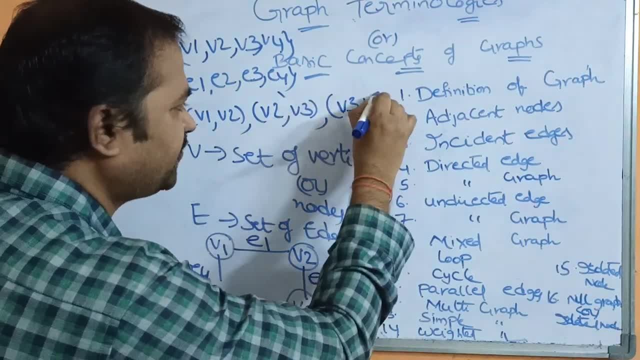 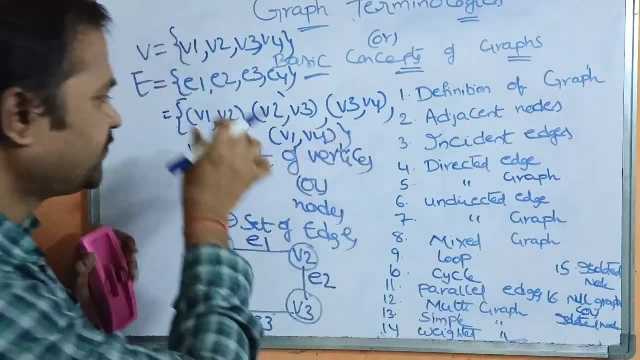 edge between v3, v4.. So v3 comma v4.. So what is v4? An edge between v1 and v2.. So this is called as pair, So an ordered pair. So we can denote an edge like this or like this. So this is about definition. 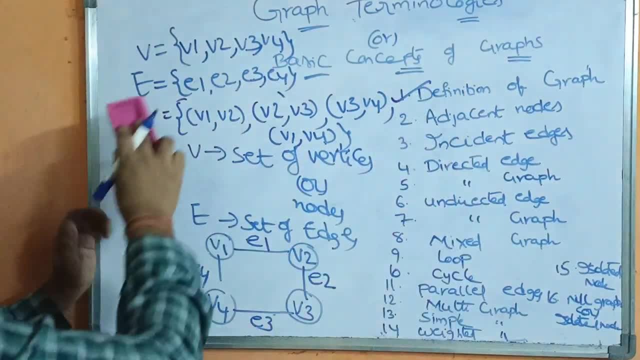 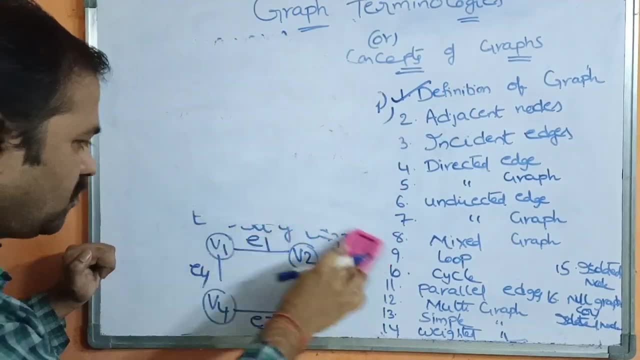 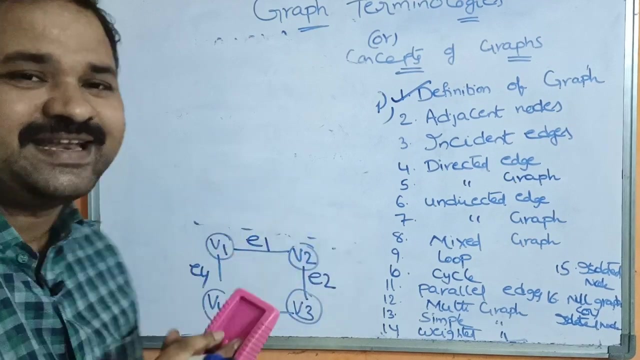 of the graph. Now let us see the second terminology. So the second terminology is adjacent nodes. So what are adjacent nodes? What are adjacent nodes, If we consider this graph? So adjacent node means If there is an edge between two nodes, then we can call them as adjacent nodes. So if 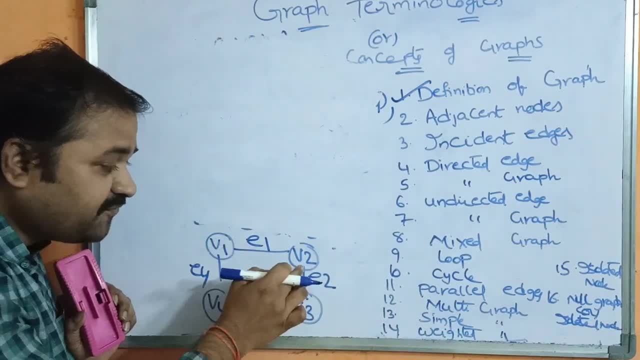 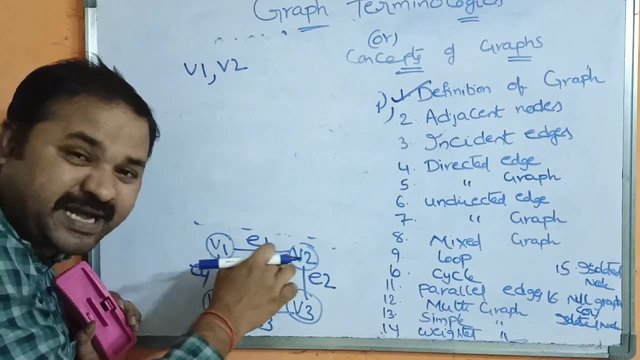 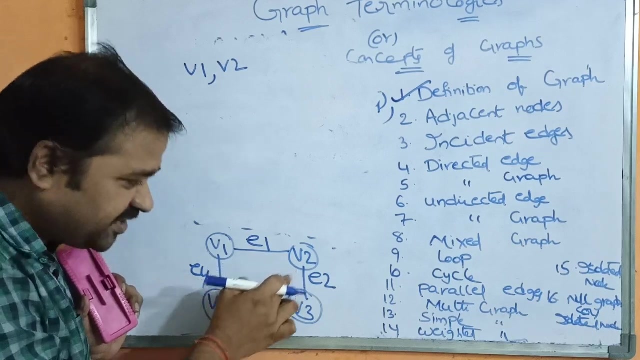 we consider this graph. Here there is an edge between v1 and v2.. So we can call v1, v2 as adjacent nodes. So what is edge? Edge is nothing but a path, A path between two nodes, If we consider v2 and v3. Here there is an edge, There is some connection between. 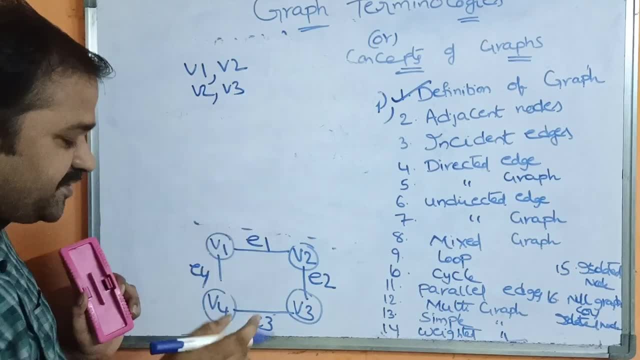 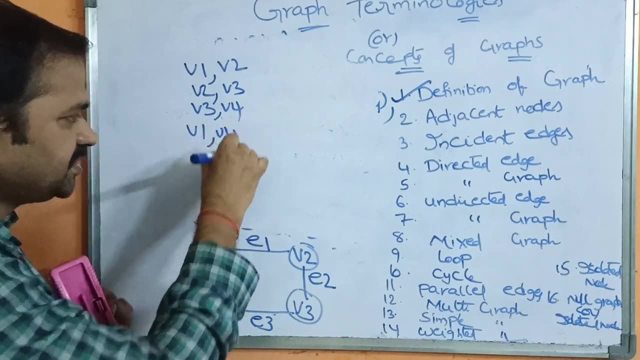 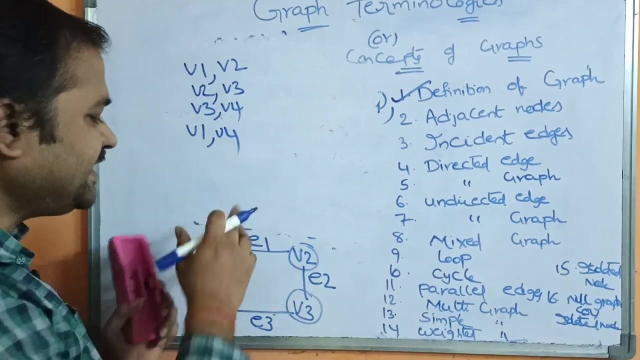 v2 and v3.. So we can call v2 and v3 as adjacent nodes. v3- v4- he has adjacent nodes. v1- v4- he has adjacent nodes. so adjacent nodes means if there is a connection between two nodes, then we can call them as adjacent nodes. there is no difference between. 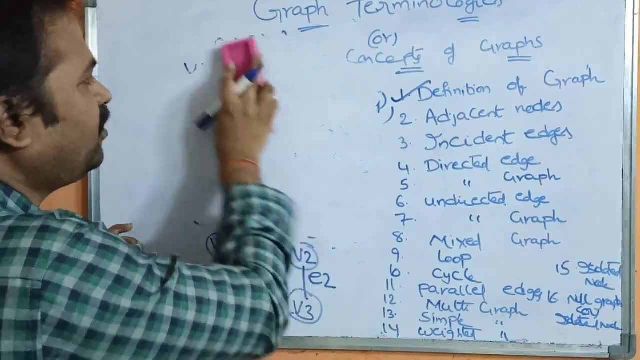 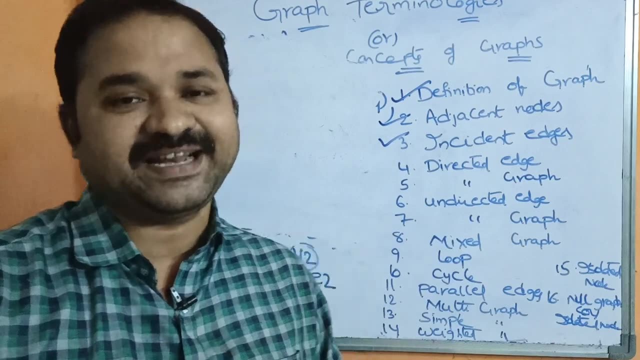 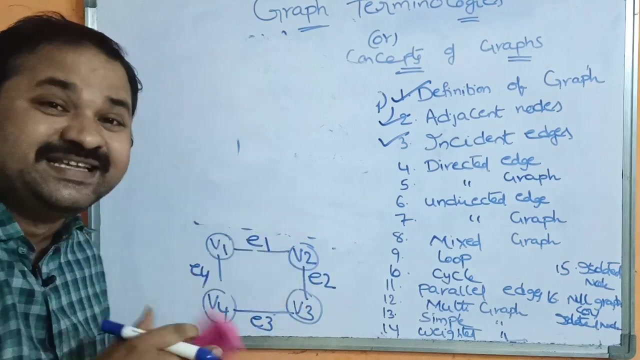 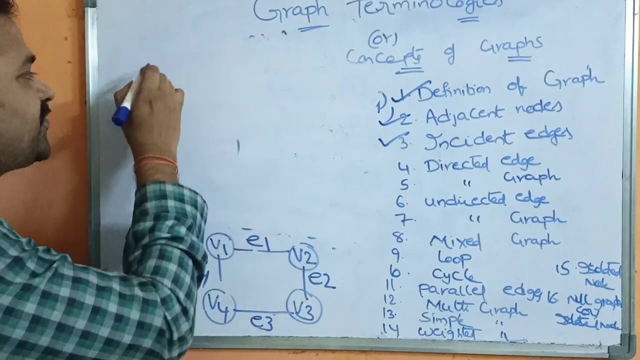 node and vertex. so both are same. only now let us see the next terminology. the next two terminology is incident edges. so what is incident edge? so an edge, an edge which joins two nodes, is called as incident edge. here this edge, e1, joins two vertices, v1 and v2, so we can call: 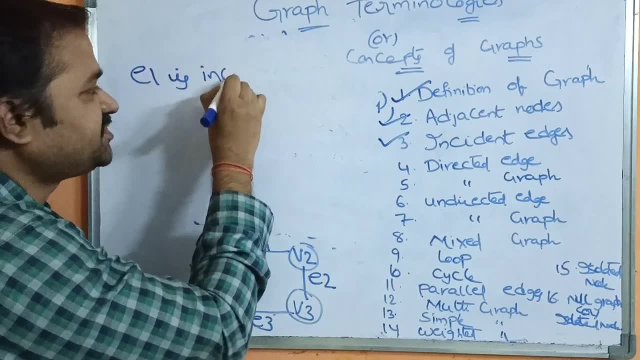 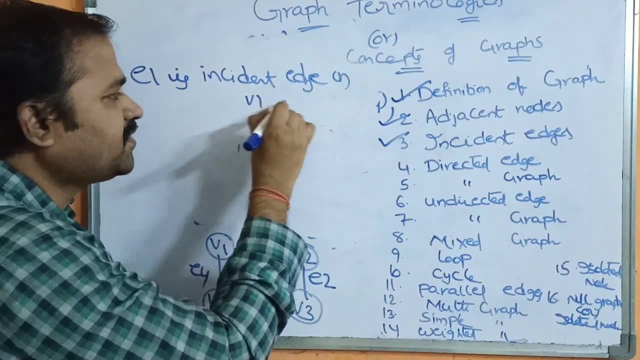 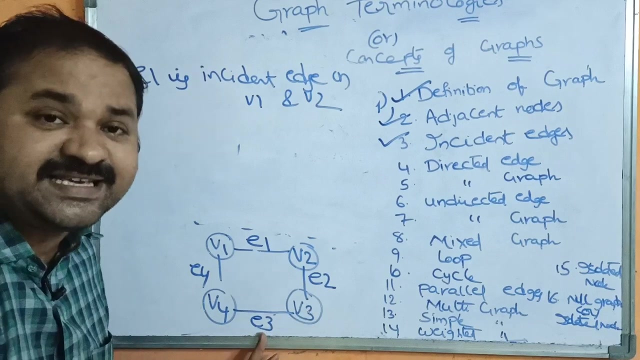 e1 as e1 is incident edge, incident edge on which vertices e1 joins v1 and v2 on v1 and v2. so likewise, e2 is incident edge on v2 and v3. e3 is incident edge on v4 and v3. e4 is incident. 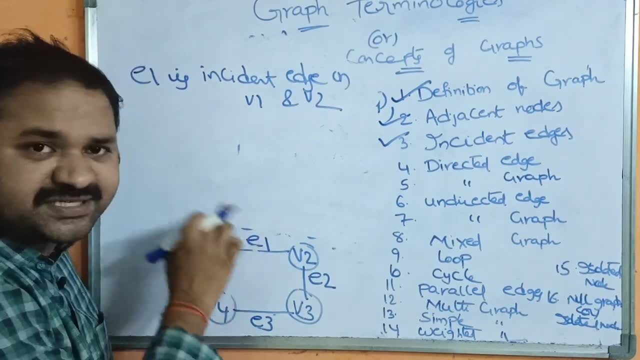 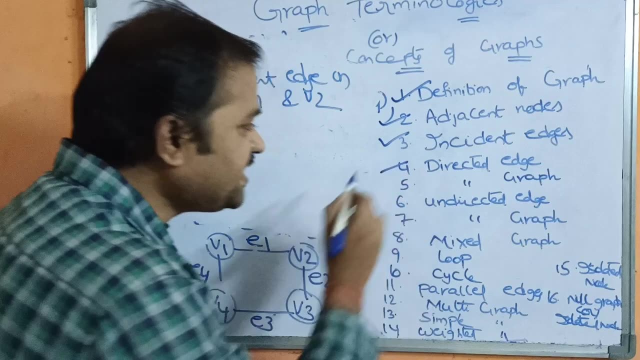 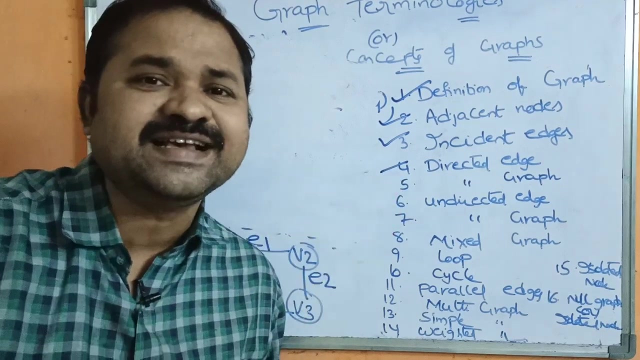 edge on v1 and v4. so if an edge joins two vertices or two nodes, then we can call that edge as incident edge. next let us see about directed edge. so what is directed edge? so directed edge means in a graph, g is equal to v comma. 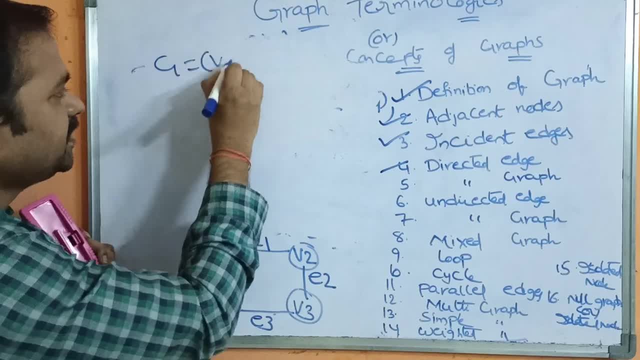 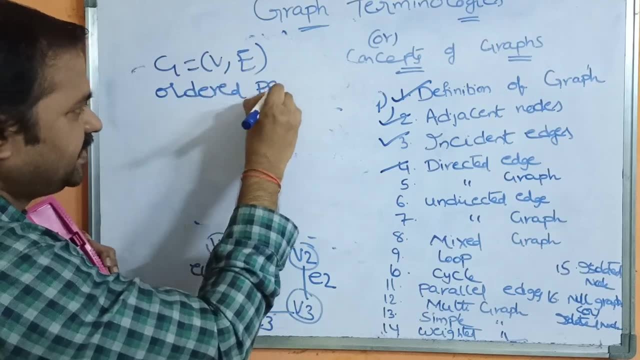 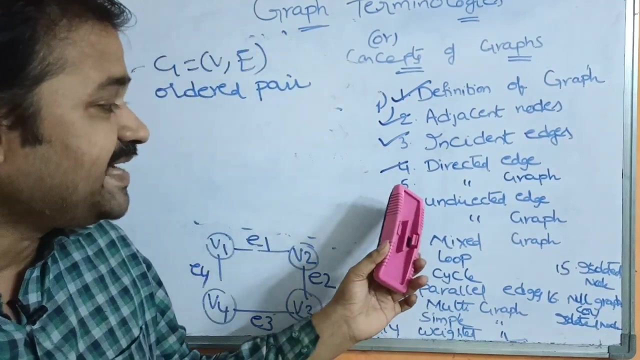 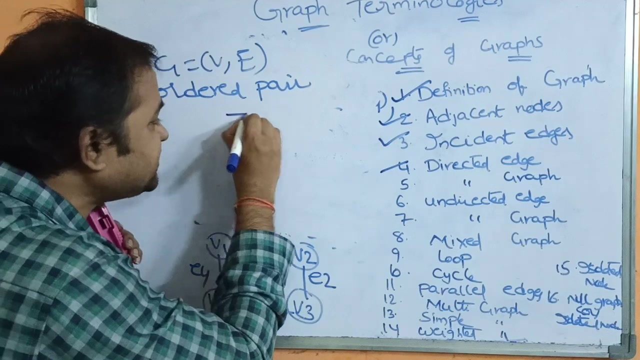 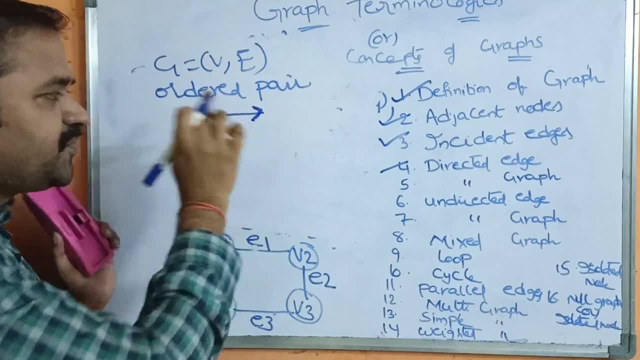 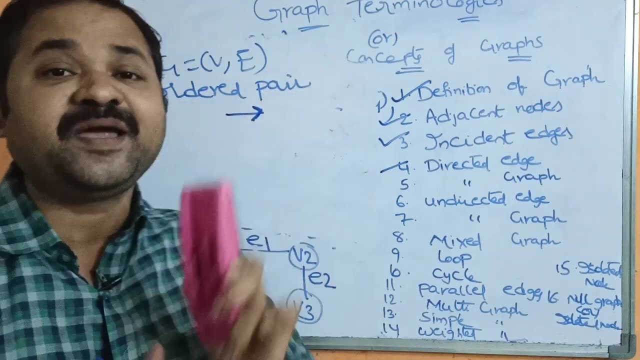 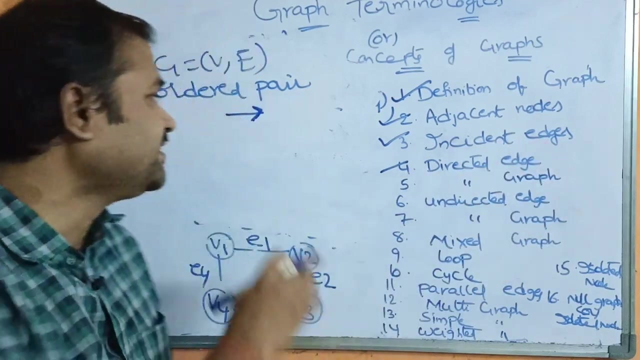 contains some direction. so here we have a direction. so this type of edge is called as directed edge. so we have two definitions, are there? if an edge contains ordered pair of vertices, then we can call that edge as directed edge. or an edge which contain some direction is called as. 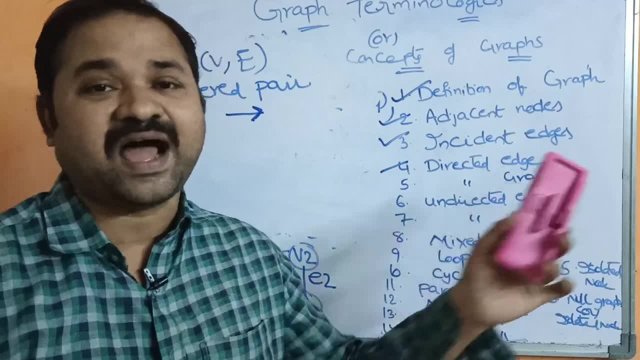 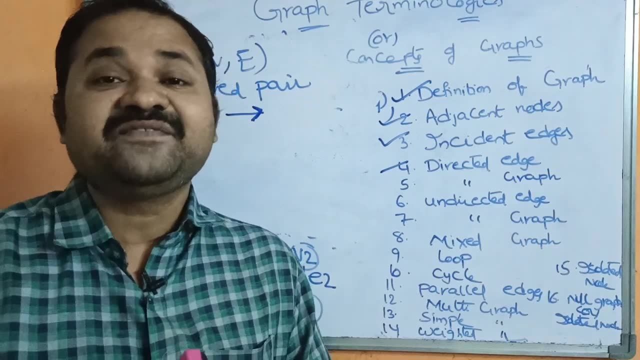 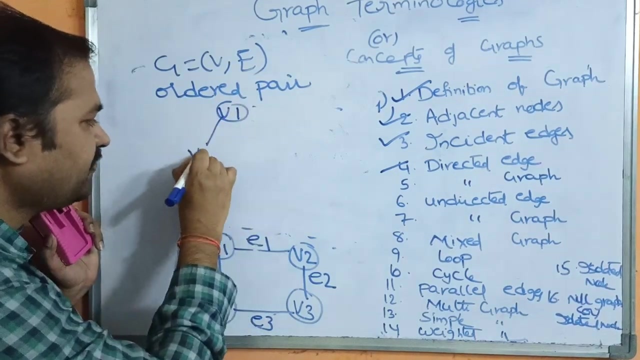 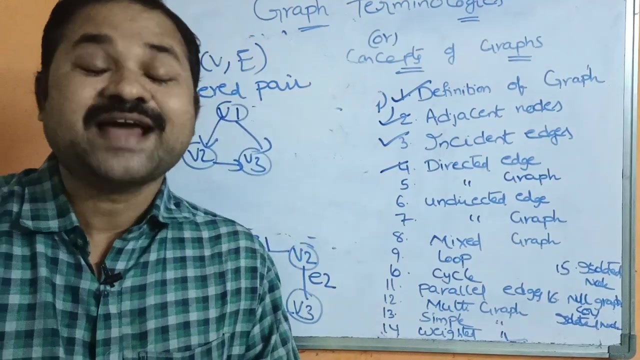 directed edge. now let us see about directed graph. so what is directed graph? if every edge in the graph is directed edge, then we can call that graph as directed graph. so let us take an example for this. so v1, v2, v3, this graph is called as directed edge directed graph. why? because every edge in the graph is 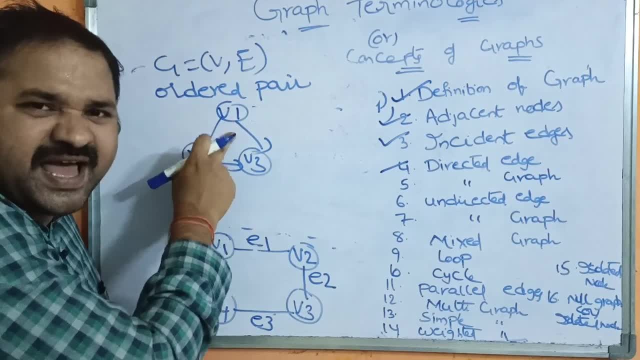 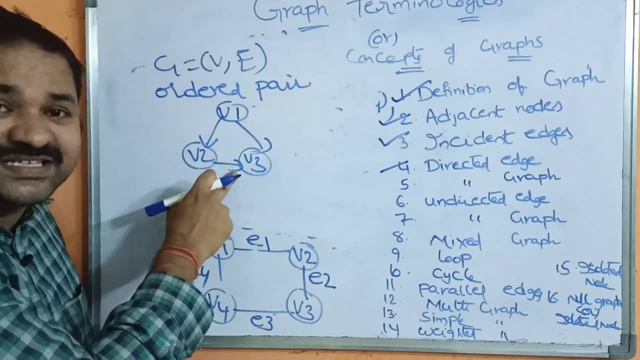 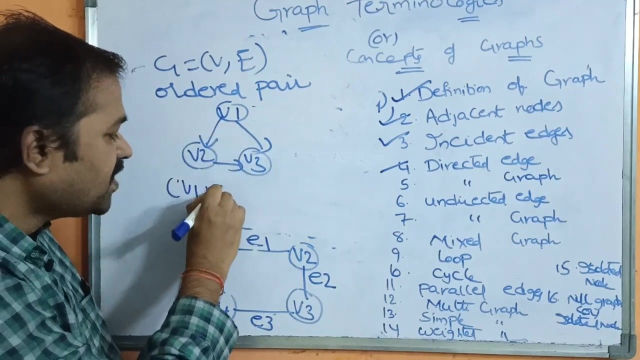 directed edge. so the here. what is directed edge? an edge which contain direction. so from v1 to v3: an edge contain direction. v2 to v3: an edge contain some direction. v1 to v2: an edge contain some direction. so here, what are the edges? here we have an edge from v1 to v3. 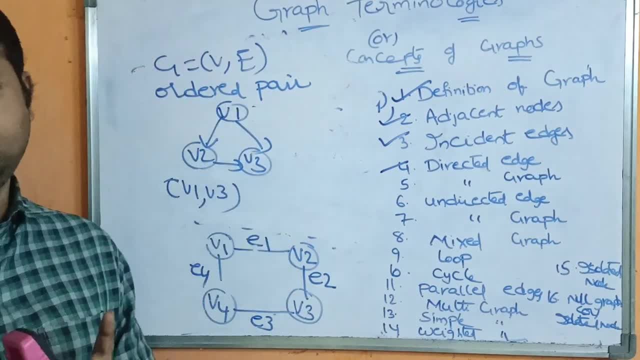 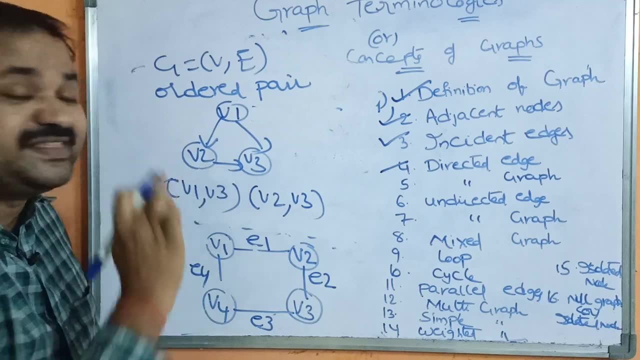 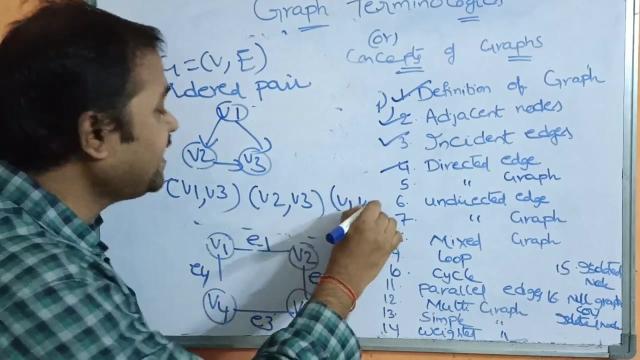 but we don't have an edge from v3 to v1. okay, next here we have an edge from v2 to v3, but we don't have an edge from v3 to v2. next we have an edge from v1 to v2, v1 to v2, but we don't have an edge. 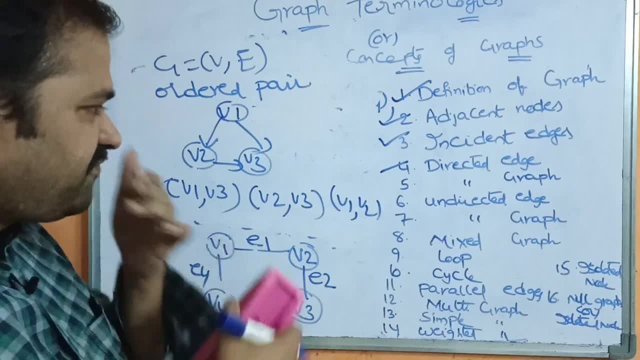 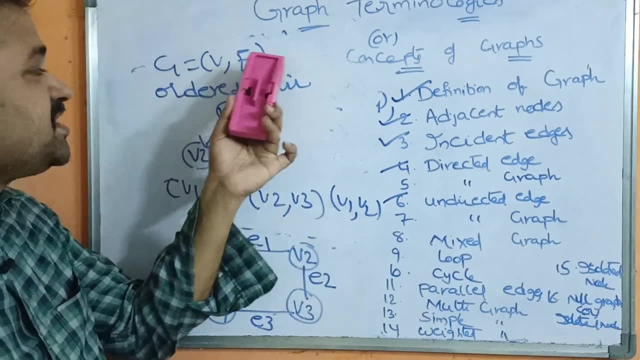 from v2 to v1. okay, that is about directed graph, undirected edge. And let us see about undirected edge. So what is undirected edge? In a graph, G is equal to V, E If an edge is associated with unordered pair of vertices. 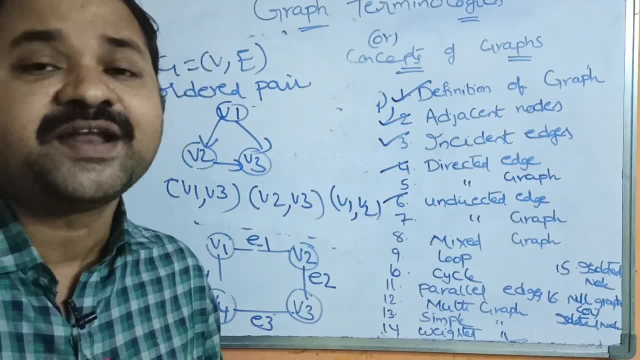 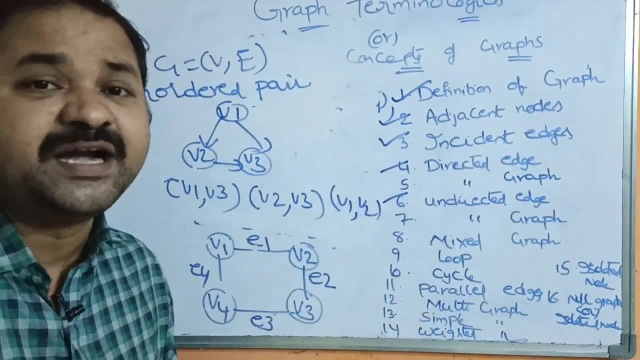 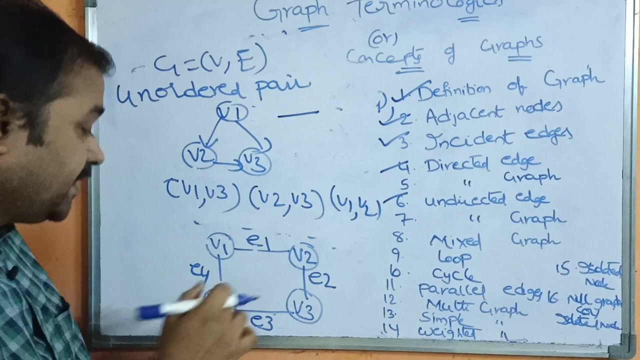 If an edge is associated with an unordered pair of vertices, Then it is called as undirected edge. So what is unordered pair? Unordered pair means that edge do not contain any direction. There is no order If we consider this graph. 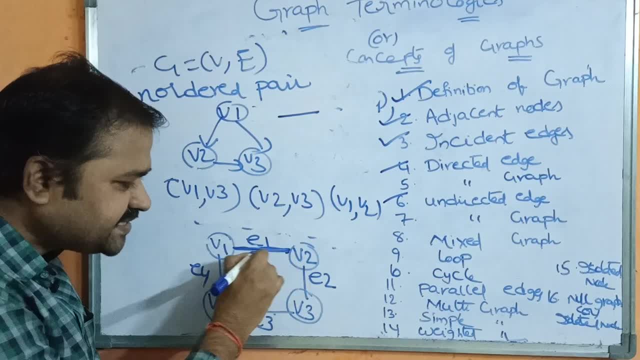 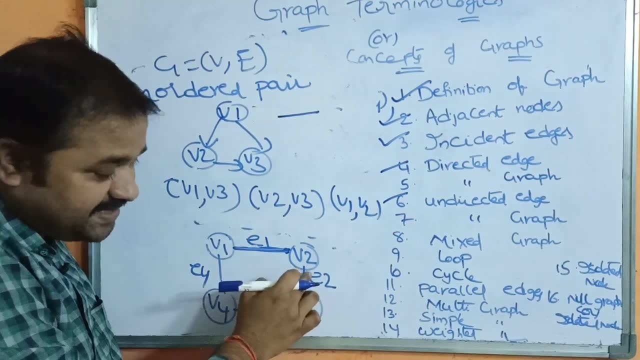 So this graph, In this graph, this edge is called as undirected edge. Why? Because this edge doesn't contain any direction. So this edge is called as undirected edge. Why? Because this edge doesn't contain any direction. 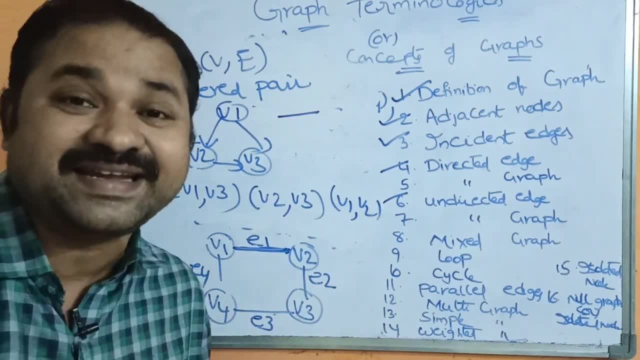 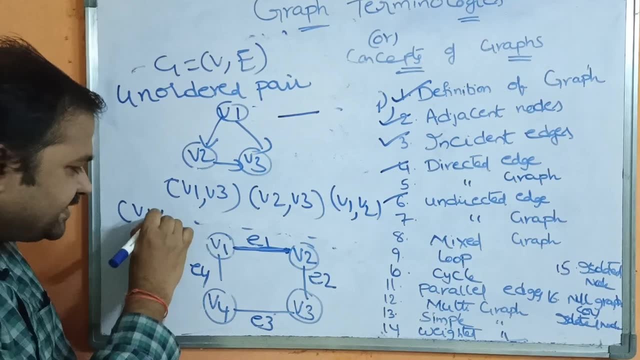 So, likewise, this edge- and this edge are also called as undirected edge, So there is no direction. So here, if there is an edge like this, Then we can say that there is an edge from V1 to V2.. Yes, 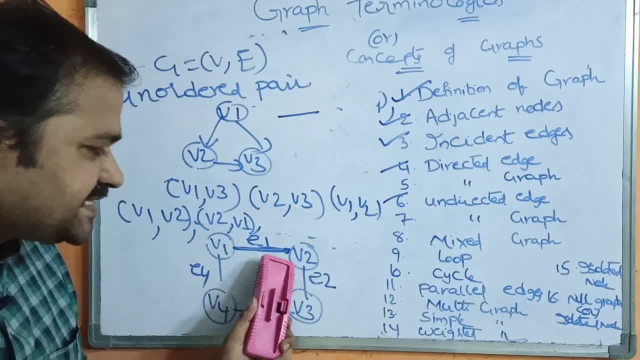 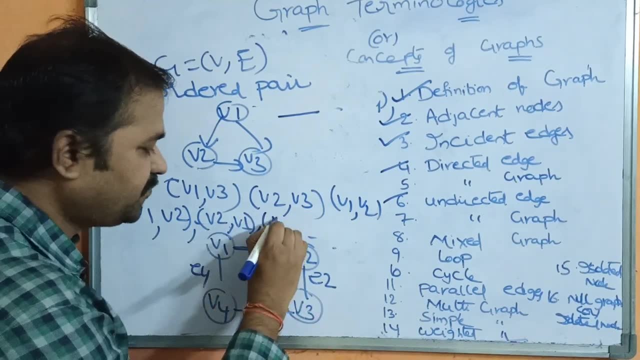 As well as there is an edge from V2 to V1.. Likewise, if there is an edge from V2 to V3. Then we can also say that this is an edge from V3 to V2.. So V2 to V3 as well as V3 to V2.. 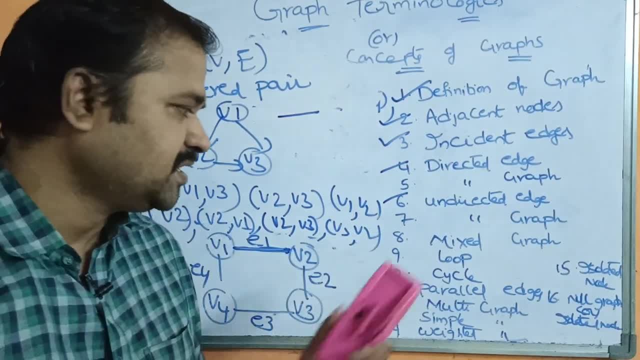 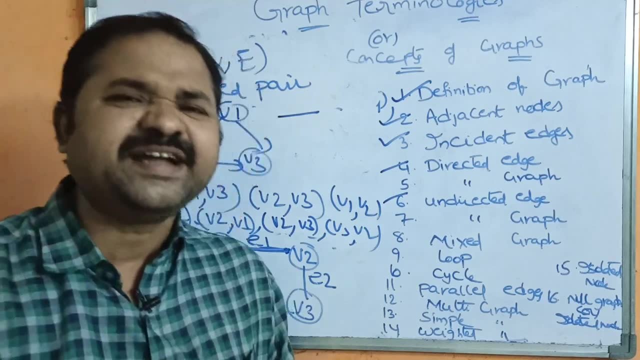 We have an edge, So likewise we have remaining edges also. Let us see about the next terminology: Undirected graph. Undirected graph means if every edge in the graph is undirected edge, Then the graph is called as undirected graph. 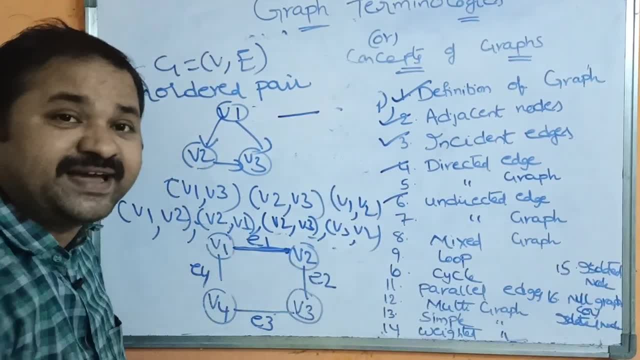 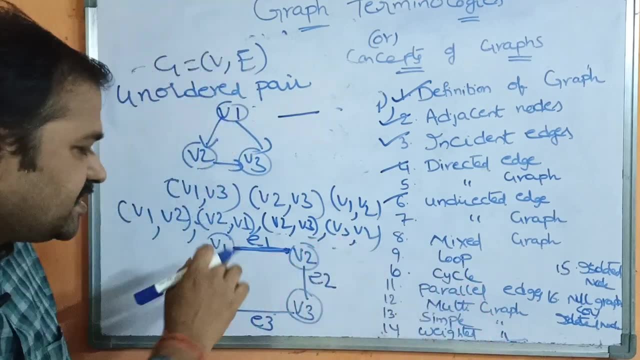 If you consider this graph, In this graph, these four edges are undirected edges only. So we can call this graph as undirected graph. Why? Because every edge do not contain any direction here. Let us see about the next terminology. 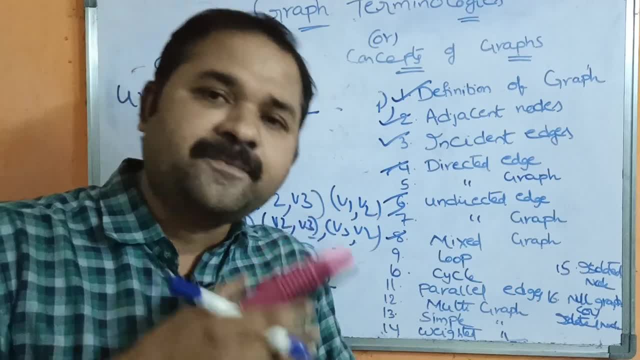 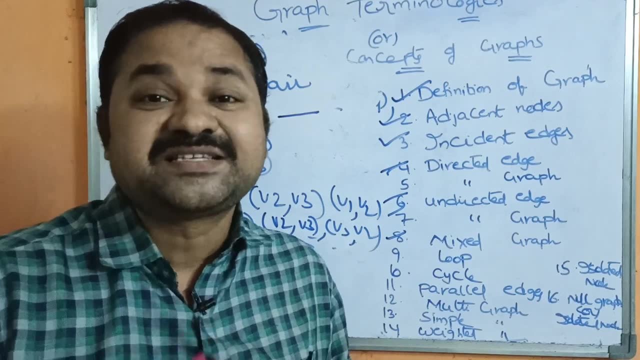 That is mixed graph. Mixed graph means if some edges are directed edges And some edges are undirected edges, Then we can call that graph as mixed graph. So let me have. Let me have undirected edge As well, as in this graph. 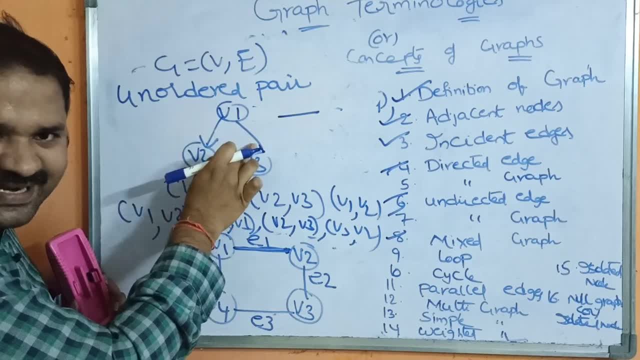 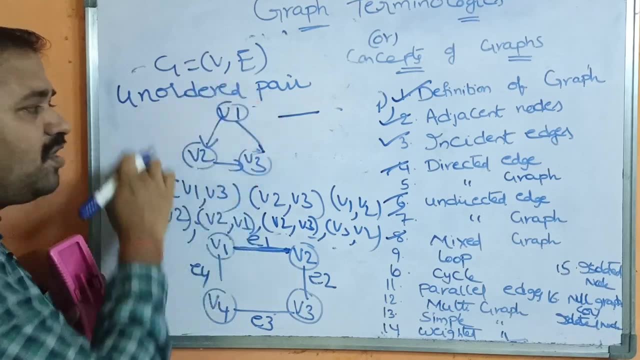 This is nothing but undirected edge. Why? Because this edge does not contain any direction, Whereas these two edges are nothing but directed edges. Okay, Directed edges, So we can call this graph as mixed graph. Mixed graph means some of the edges are directed edges. 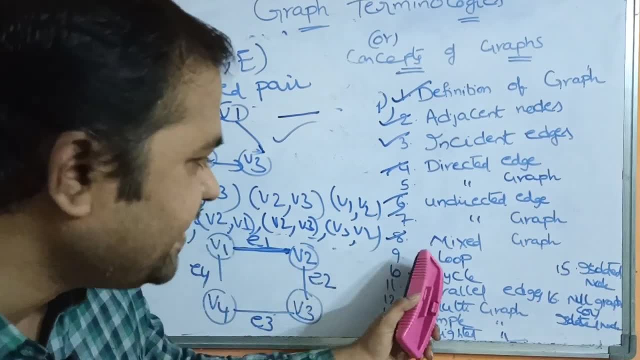 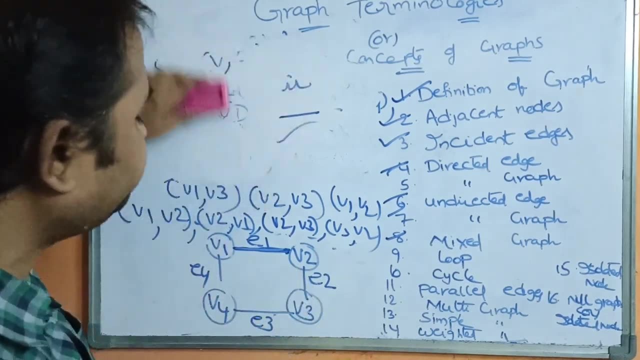 And some of the edges are undirected edges. Let us see the next terminology. The next terminology is loop. So what is a loop? Loop is nothing but an edge where the starting and ending vertex are the same. So what is loop? 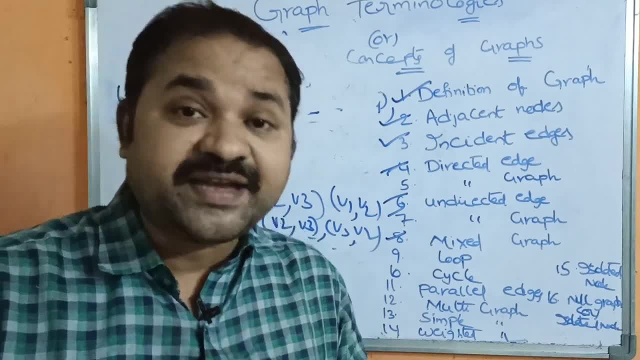 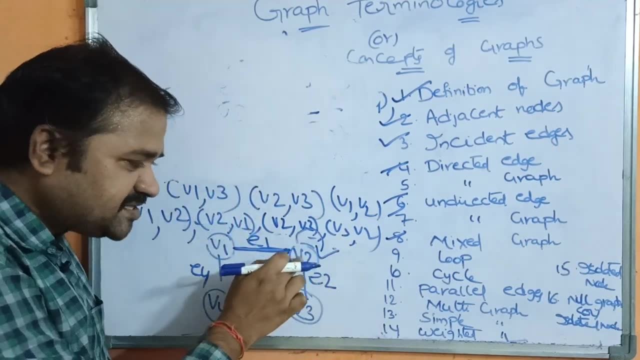 Loop means an edge where the starting vertex and the ending vertex are the same. So this is a loop. This is a loop. Why? Because here this is an edge where the starting vertex is v2.. As well as the ending vertex is v2.. 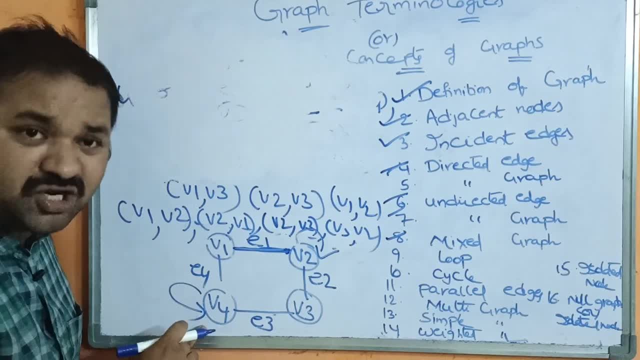 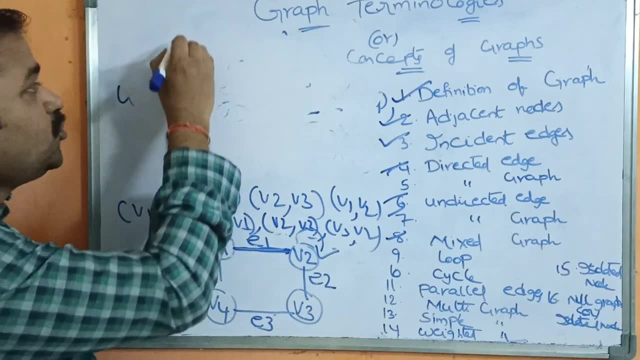 Okay, Let us take this one. This edge is also loop. Why? Because here the Starting vertex is v4.. As well as ending vertex is also v4. So for the loop the starting and ending vertex are same only. 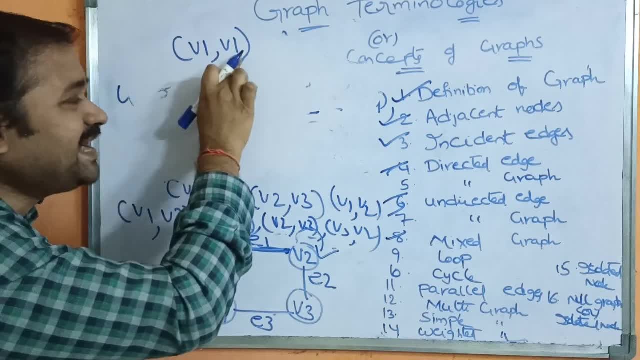 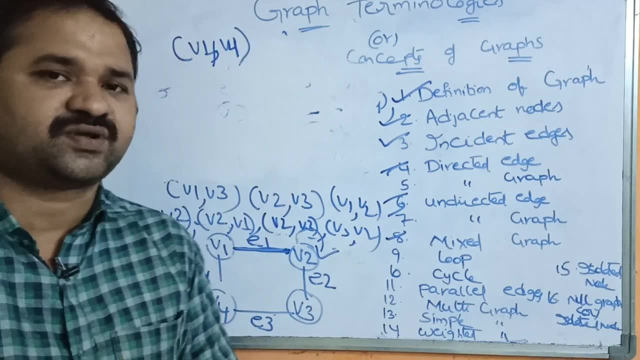 If the starting vertex is v1, then ending vertex should also be v1. only If the starting vertex is v4, then ending vertex should also be v4.. Next let us see about cycle. Loop means we will have only one edge. 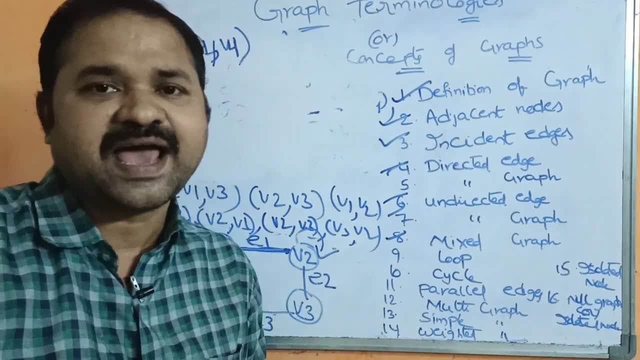 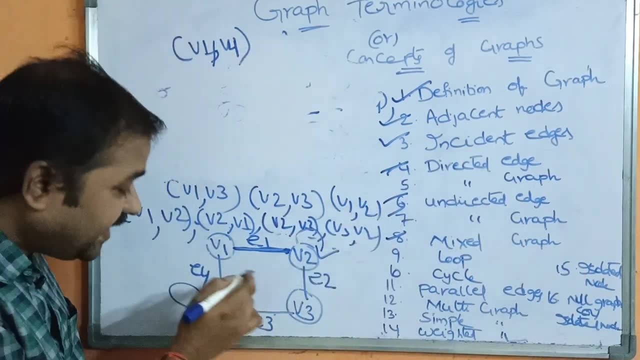 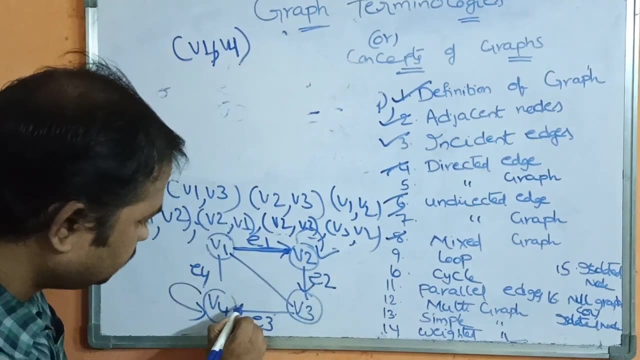 Various. cycle means a set of edges. Cycle means a collection of edges where the starting vertex and the ending vertex are the same. If we consider this graph let, this is a directed graph- a directed graph. So, if we consider this graph, this graph contains a cycle. 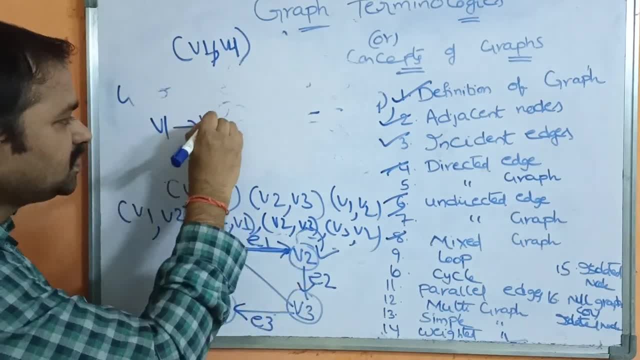 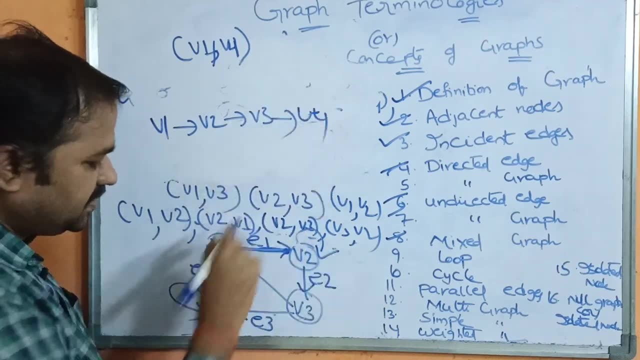 From v1, we can go to v2.. From v2, we can go to v3.. From v3, we can go to v4.. From v4, we can go to v1.. So this is a cycle. 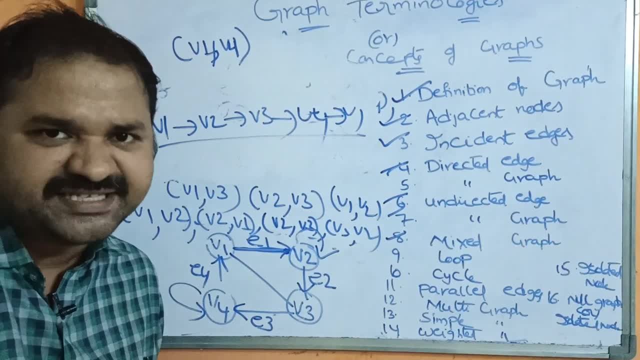 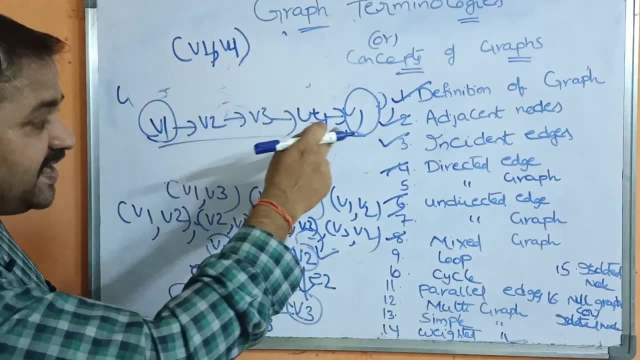 Why? Because what is a cycle? Cycle means a collection of edges where the starting vertex and the ending vertex are same. Here, the starting vertex is v1, as well as ending vertex is also v1.. So, likewise, if we consider v2.. 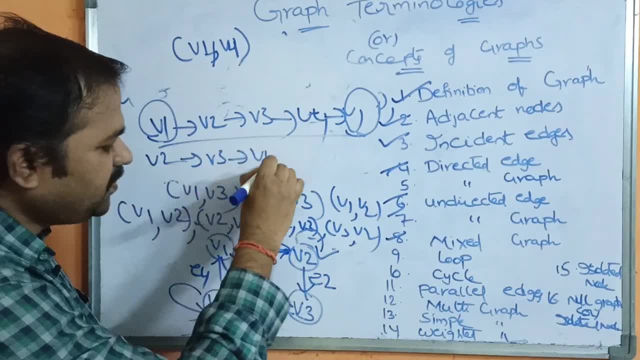 So from v2, we can go to v3.. From v3, we can go to v4.. From v4, we can go to v1.. From v1, we can go to v2.. This is another cycle. 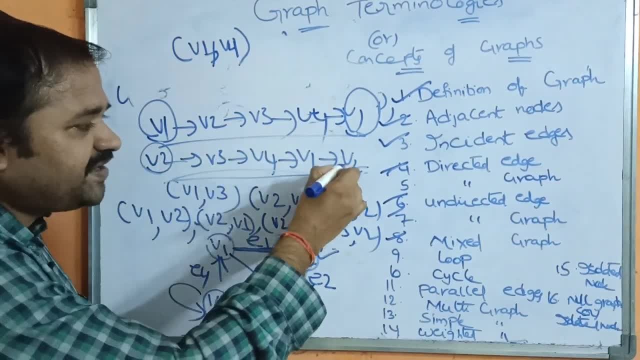 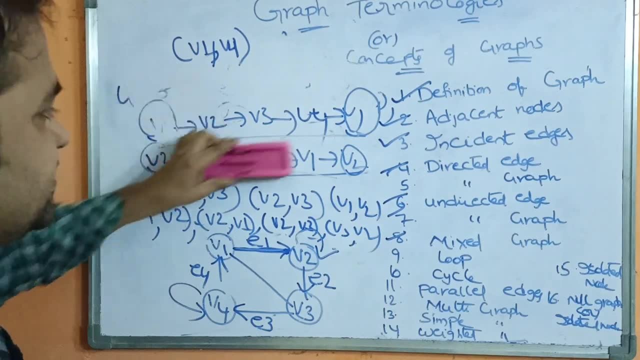 Why? Because cycle means A set of edges where the starting vertex and the ending vertex are the same. Let us see about the next one. The next one is parallel edges. So what are parallel edges? So let us consider a graph like this: 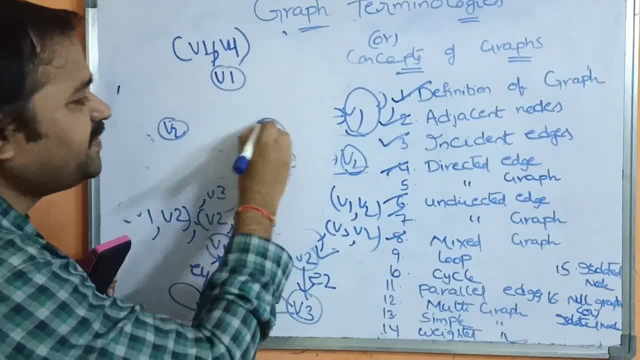 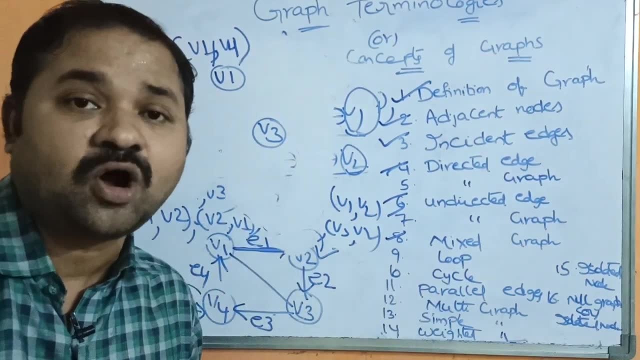 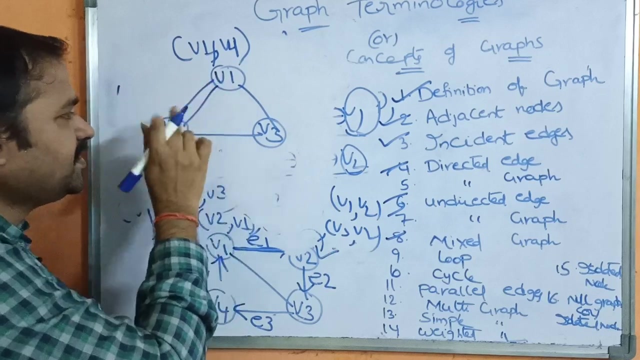 So v1, v2, v3.. Parallel edge means if there is more than one edge between a pair of vertices, then those edges are called as parallel edges. If we consider this graph, If we consider this graph, Let us take one more edge here. 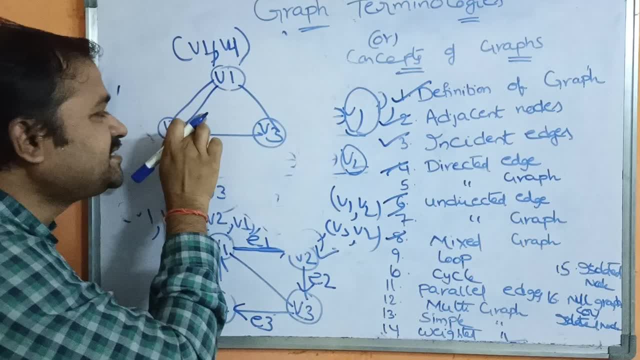 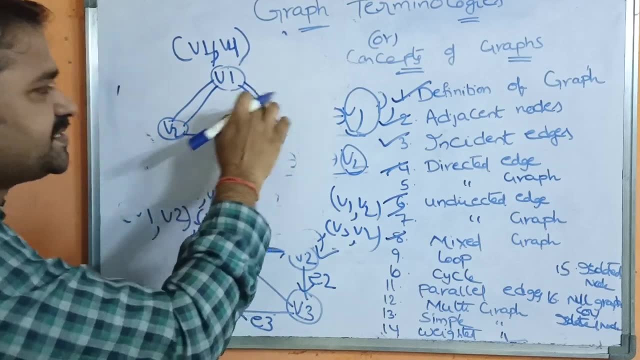 From v1 to v2, we have two edges, So these two edges are called as parallel edges. Let us consider one more edge. From v1 to v3, we have two edges, So these edges are called as parallel edges. 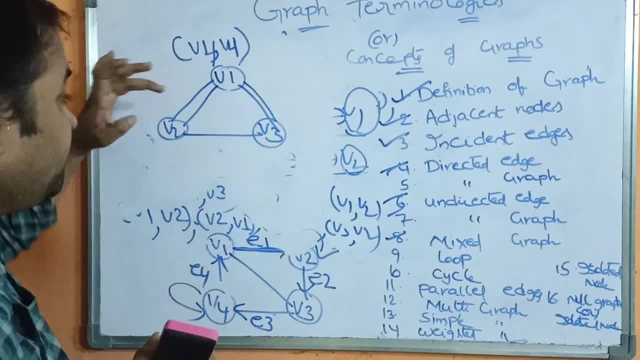 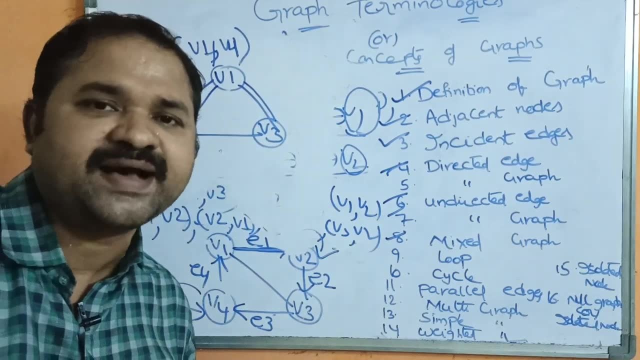 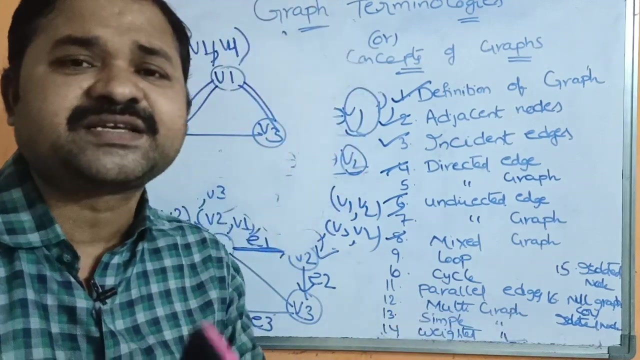 So what are parallel edges? If there is more than one edge between a pair of vertices, then those edges are known as parallel edges. Let us see the next terminology, That is, multigraphy. Multigraphy means if a graph contains some parallel edges, then we can say that that graph is multigraphy. 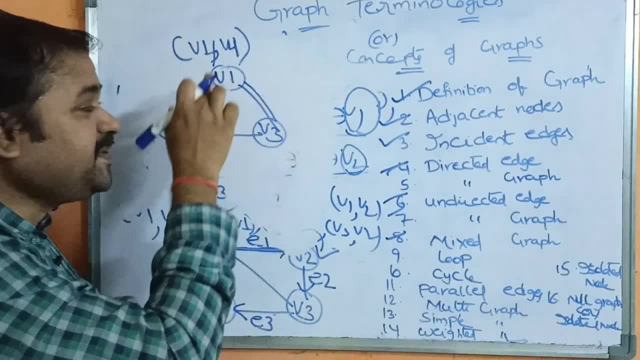 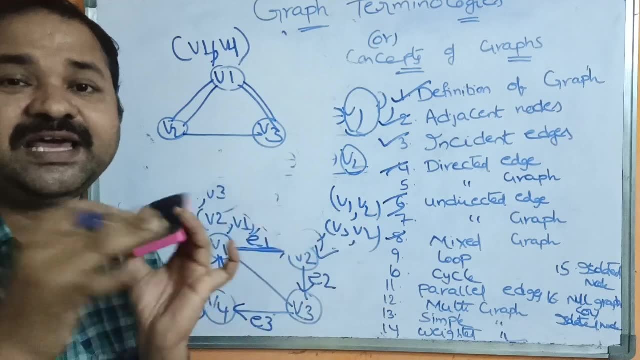 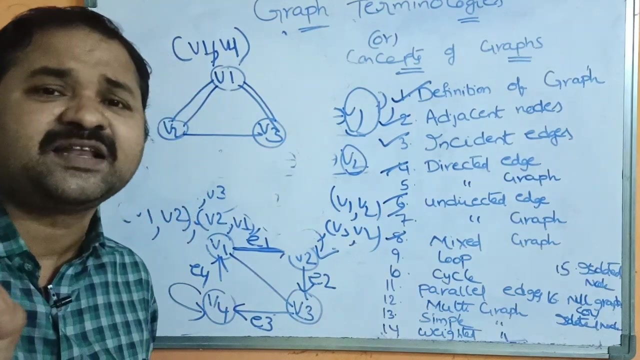 This is an example for multigraphy. Why? Because in this graph we have two parallel edges. Here all the edges need not be parallel edges. If some edges are parallel edges, Let us say we have four edges. So out of four edges, if one edge is a parallel edge, then the corresponding graph is called as multigraphy. 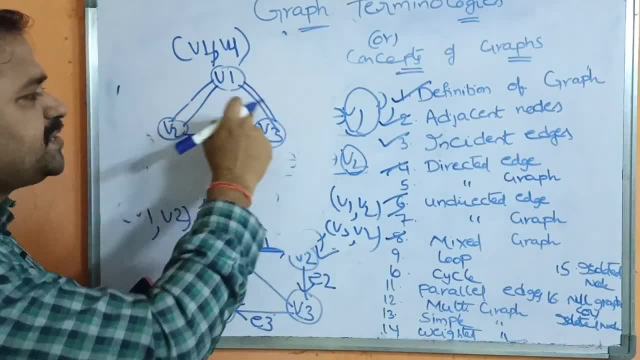 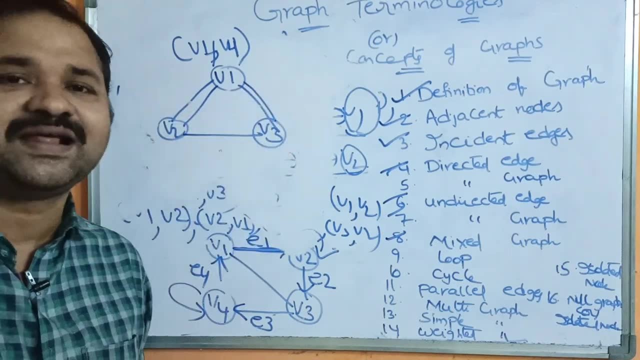 Here we have two edges. Here we have three edges: One, two, three, four. Here we have five edges Out of five edges. these two edges are parallel edges, So we can say this graph as multigraphy. 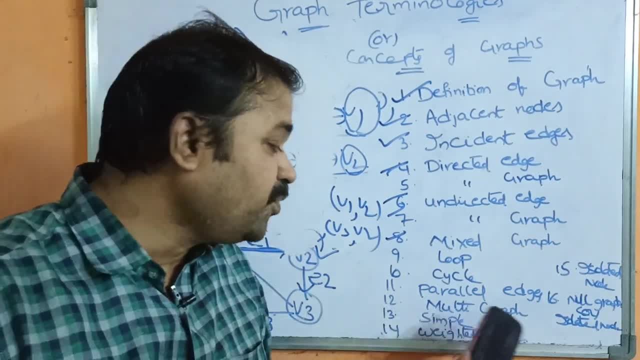 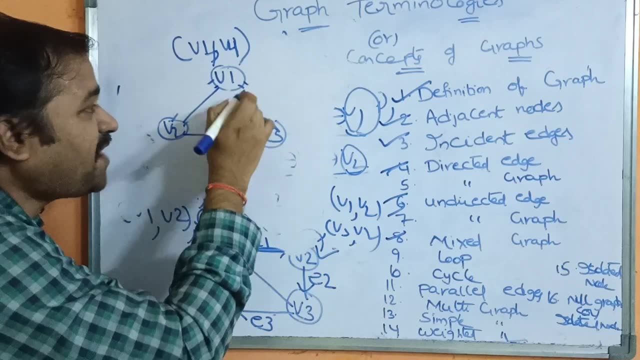 Let us see about the next one: Simple graph. Simple graph means: if a graph does not contain any parallel edges, then the corresponding graph is known as simple graph. In this graph we do not have any parallel edges, So this graph is called as simple graph. 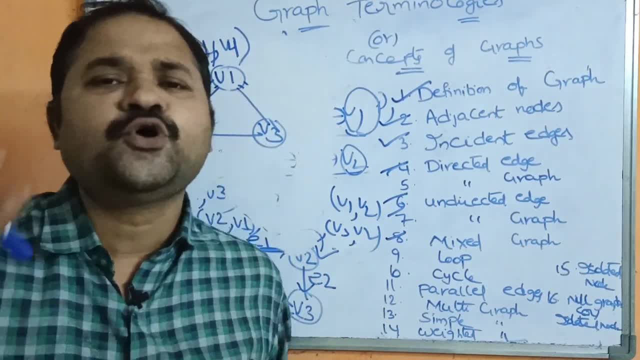 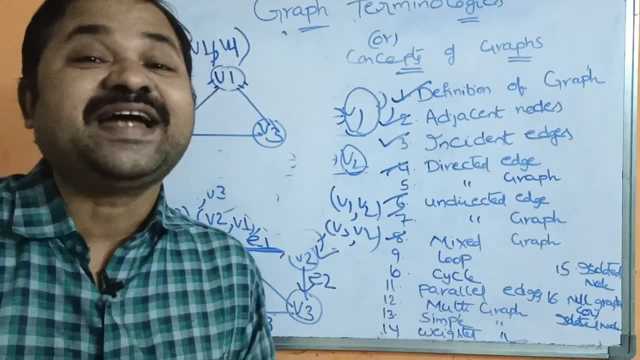 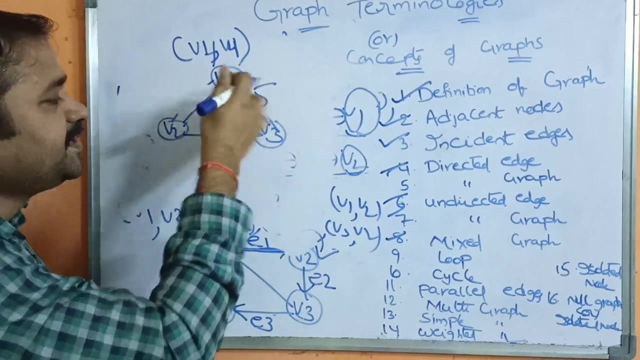 So this graph is called as simple graph. A graph with no parallel edges is known as simple graph. Let us see the next terminology: Weighted graph. Weighted graph means if every edge contains some weight, some cost, then it is known as weighted graph. 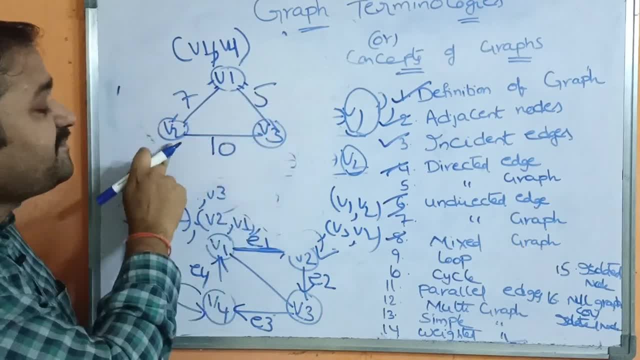 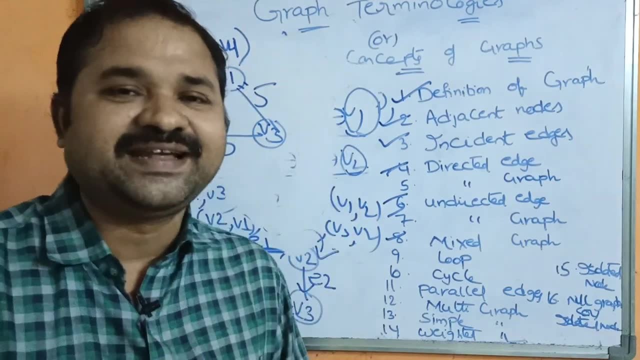 Here the weight between V1 and V3 is 5.. The weight between V2 and V3 is 10.. The weight between V1 and V2 is 7.. So this graph is called as weighted graph. If every edge contains some weight, some cost, then that graph is called as weighted graph. 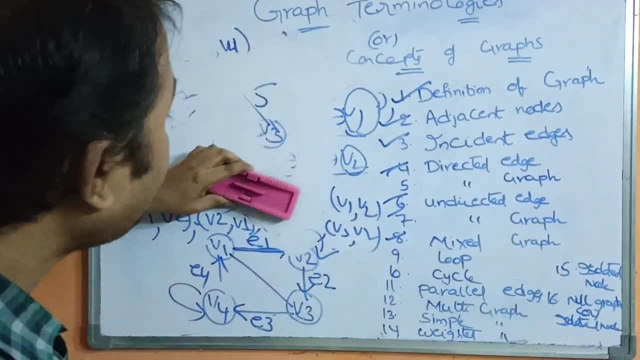 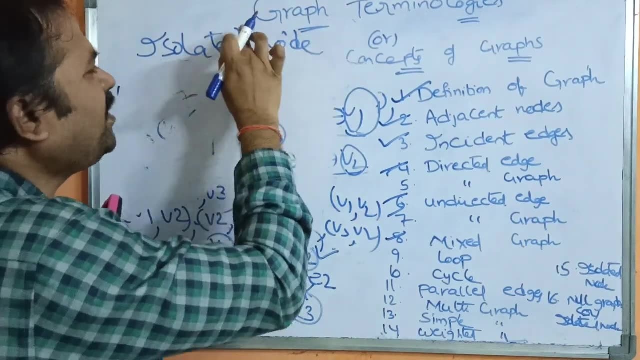 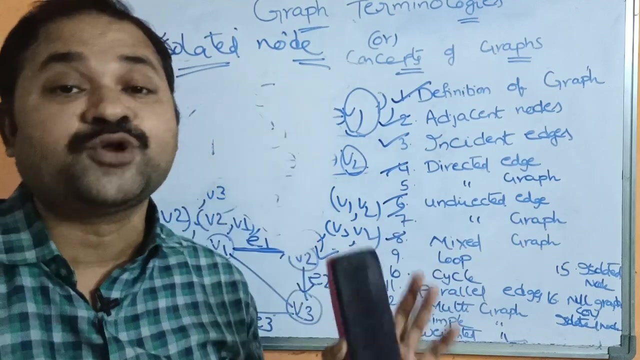 Let us see about the next one. The next terminology is isolated node. The next terminology is isolated node. Isolated node means that node is separated from the graph. That means an isolated node does not contain any adjacent nodes. That means an isolated node does not contain any adjacent nodes. 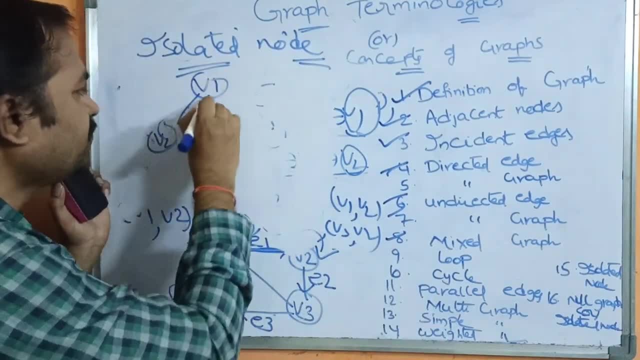 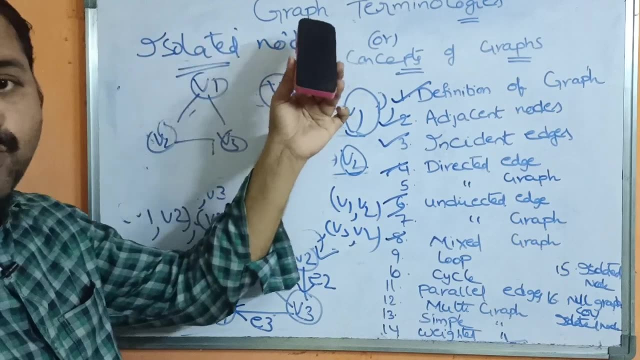 So let us have a graph like this: V1, V2, V3.. Let us have one more vertex called V4. So here V4 is called as isolated node. Why? Because V4 does not have any adjacent node. 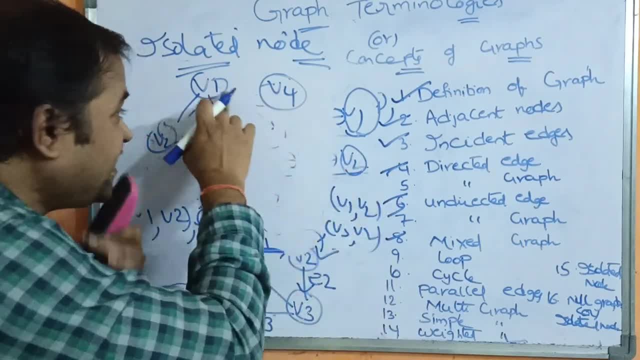 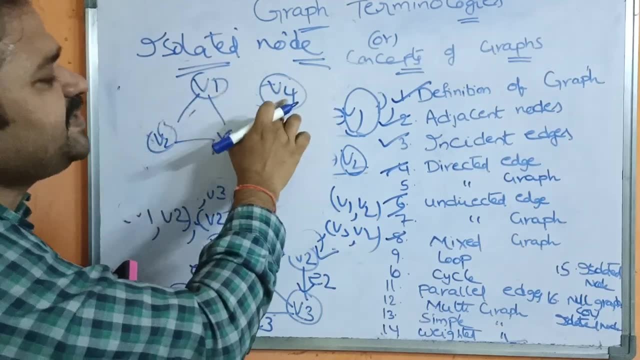 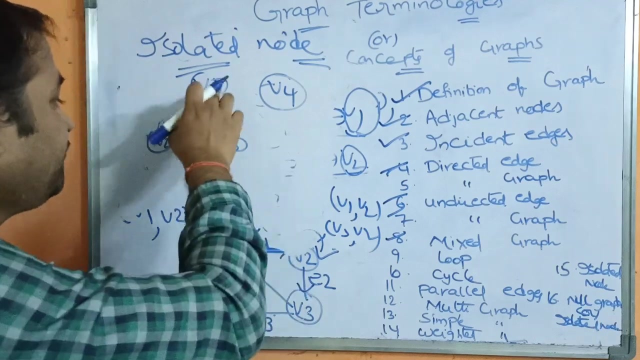 So when V4 will have some adjacent node, if there is an edge between these three nodes, whether if there is an edge between V1, V2 or V3, then we can say that those two nodes are adjacent nodes, But here from V4, we don't have any edge to V1, V2, V3. 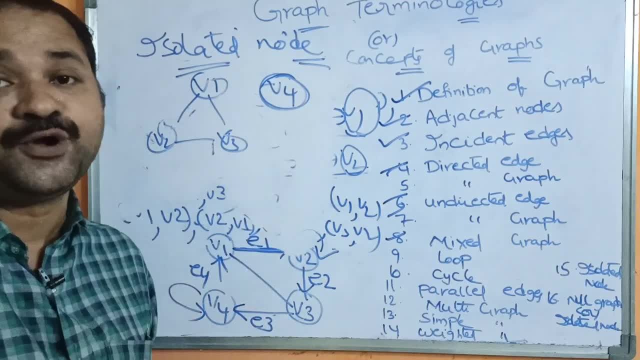 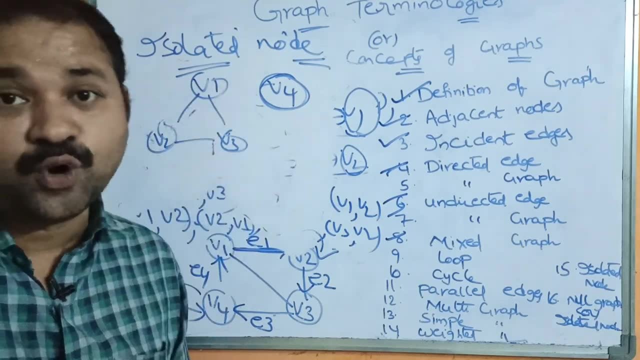 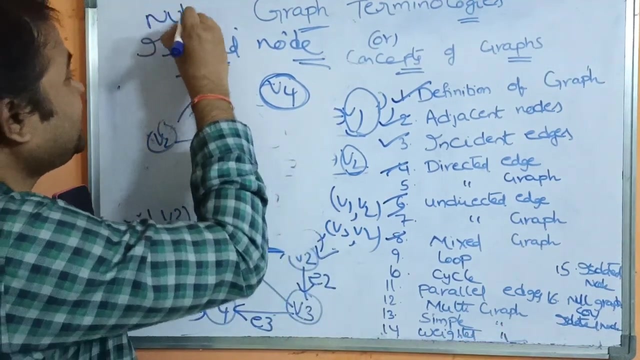 So that's why we can call this V4 as isolated node. If an edge doesn't contain any adjacent node, then it is called as isolated node or isolated vertex. Node and vertex, both are same, only- And the last terminology is null graph. 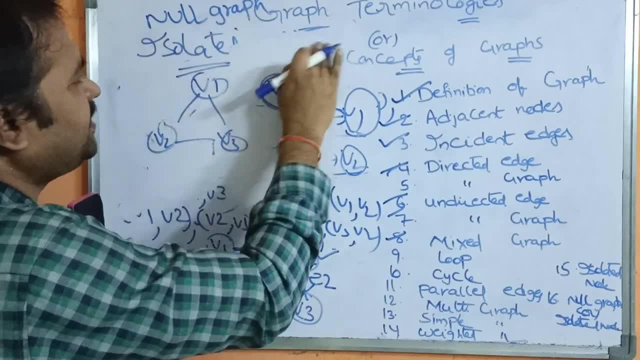 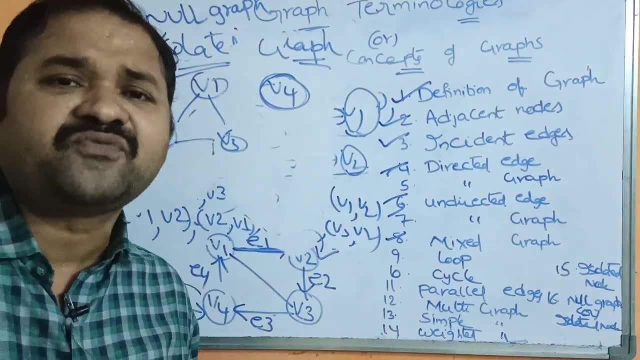 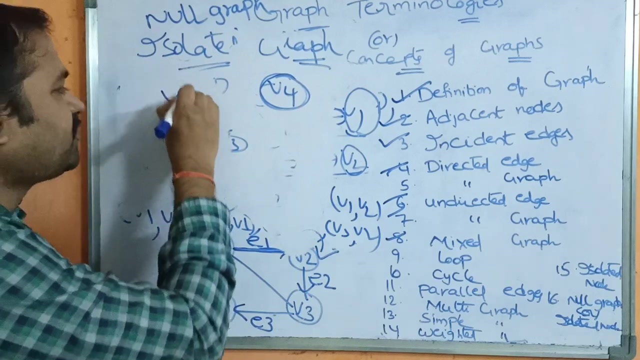 Null graph Or this graph can also be called as isolated graph. So null graph or isolated graph means if all the nodes of the graph are isolated nodes, then we can call that graph as null graph or isolated graph. So this is an example for isolated graph. 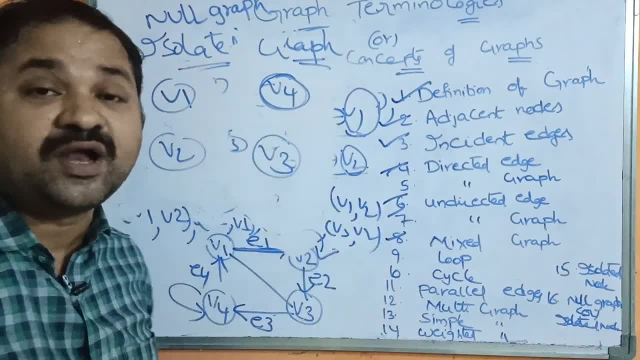 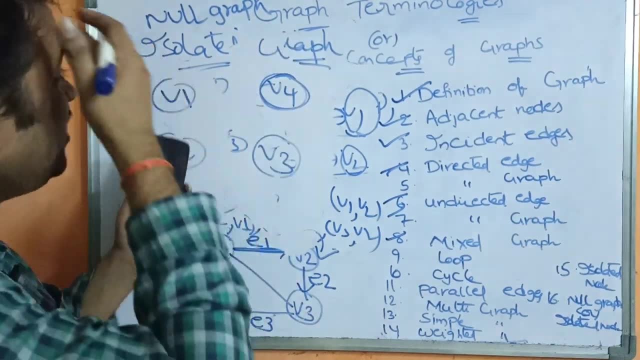 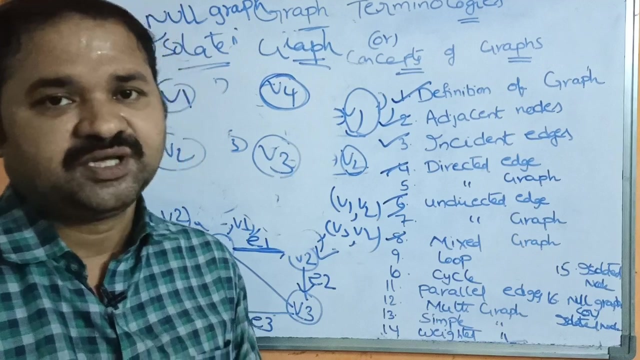 Why? Because here all the nodes are isolated nodes. only V1 is isolated node. V2 is isolated node V3 and V4 are isolated nodes. So isolated graph or null graph means in a graph if all the nodes are isolated nodes. 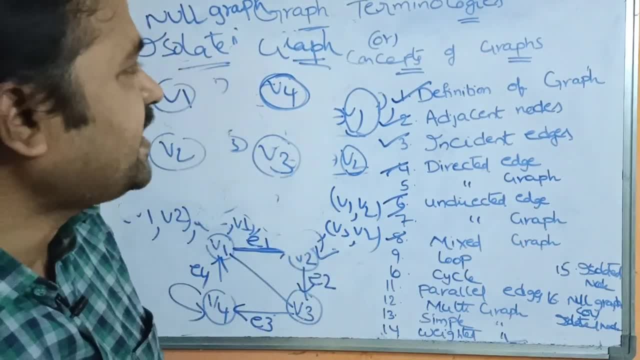 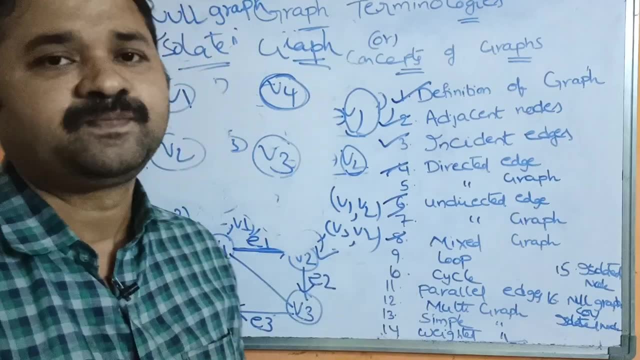 then we can call that as null graph or isolated graph. So this is about various graph terminologies or various graph concepts.